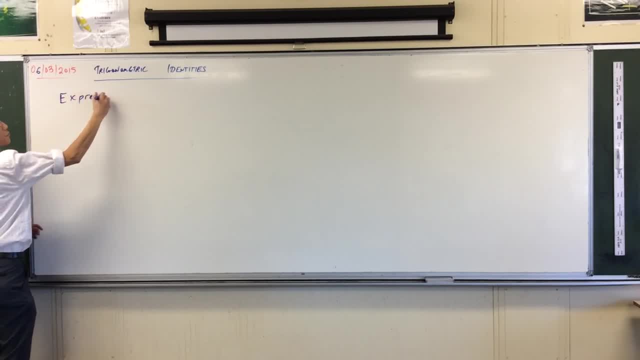 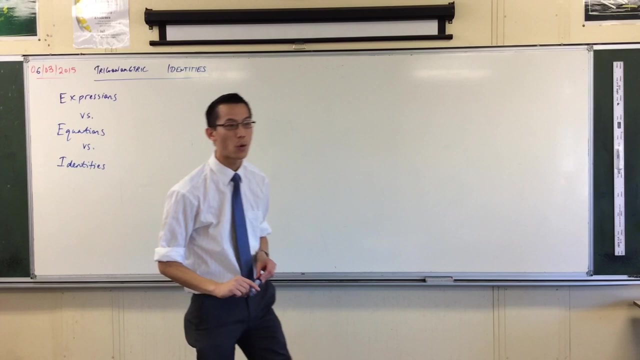 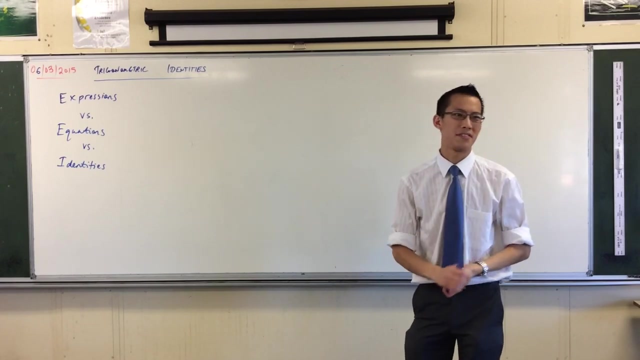 Okay, so underneath this heading, would you write for me these two things, or three things, I suppose, Because putting them in this context, I hope you understand what identities are and what they are not. So, expressions and equations: We've met these a long time ago, In fact, even as early as- oh gee, yeah, year seven. you're solving equations and you're learning what expressions are. 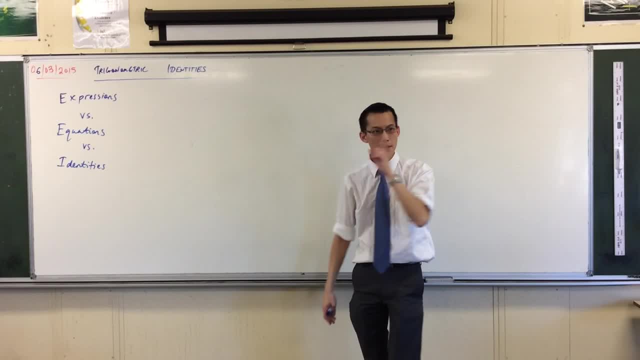 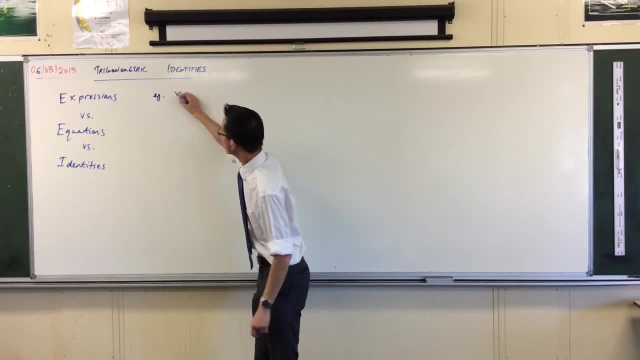 And how to collect like terms, blah, blah, blah. So what's an expression? An expression is just a collection of terms, That's all it is. So, for example, you could say x, x, squared, There you go, That's an expression. 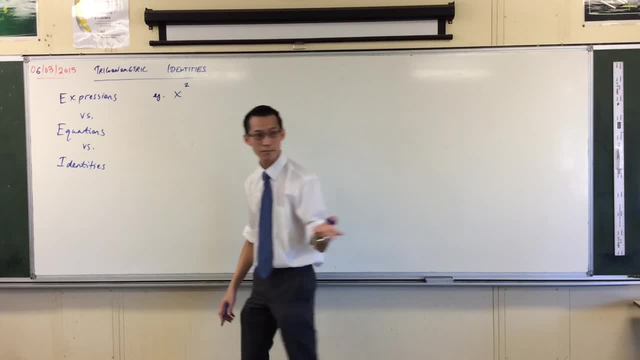 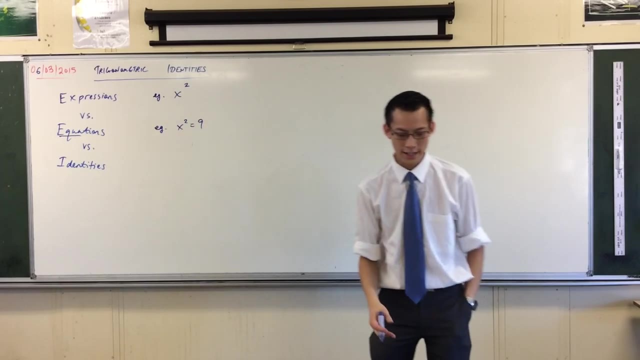 Significantly. it's not an equation because it's missing what. It's missing an equality sign, right, And equals something. So I could say an equation Which would be similar to this: is x squared equals nine, right, So it has the expression in it, But then it's saying it's equal to something else, And then you can solve it right. 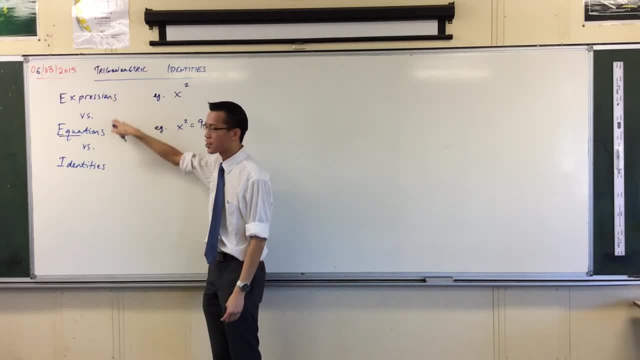 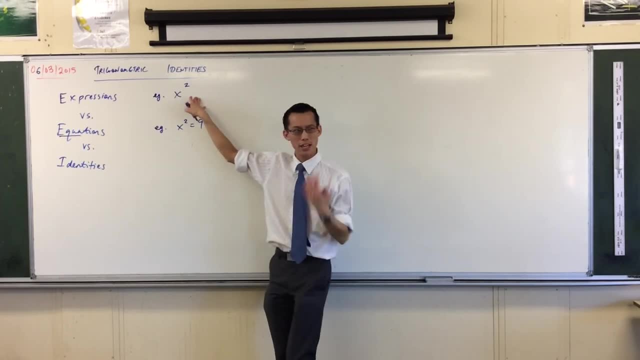 So you may remember, you can simplify expressions, but you can only solve equations. You can't solve an expression. It's not equal to anything, okay? So this is like, if you want to think about it in grammar terms, this is like a word and this is like a statement. okay, This is saying something is equal to something else. 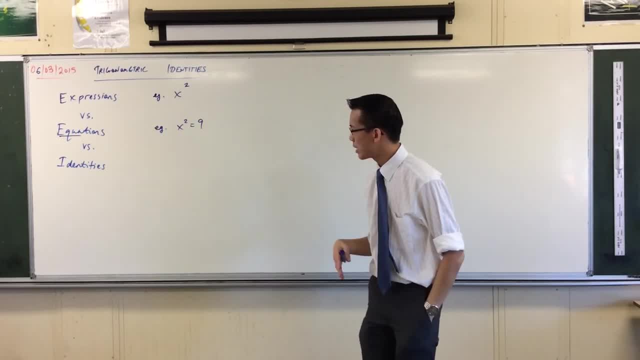 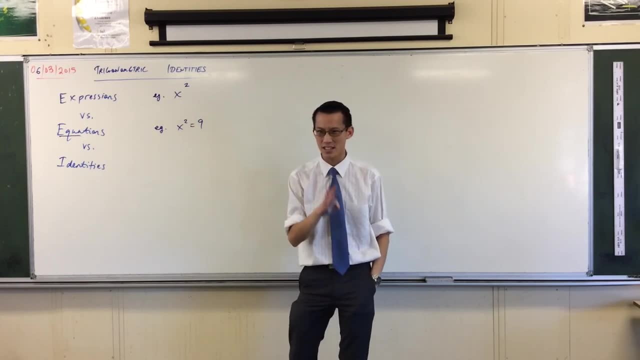 Okay, now identities- different again. It's a bit tricky because we tend to- I think partly because we're lazy- we use the same notation for identities that we do for equations, but actually there's a slightly different term you should use, So let me give you. 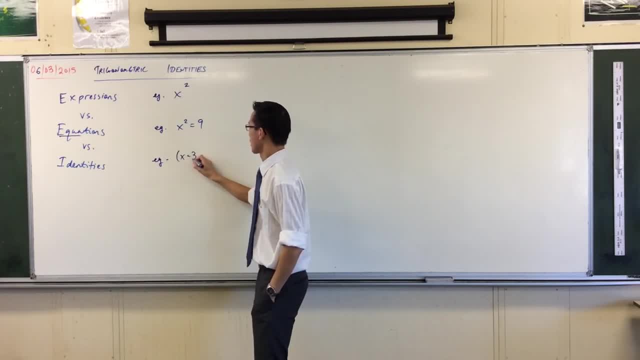 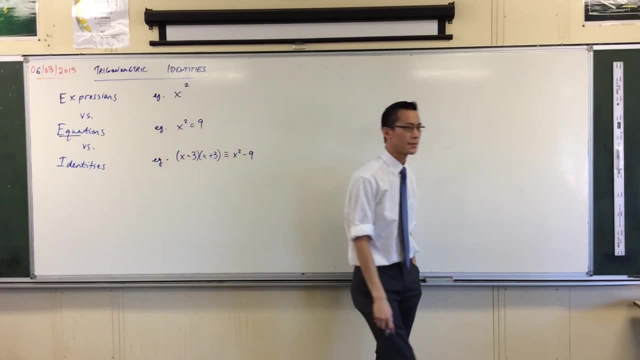 an example. Here's something. Now a couple of things. The first thing you'll notice, okay, is that this equation cannot be solved, Partly because it's not an equation. See that? Yeah, We would usually write an identity like the way you've. 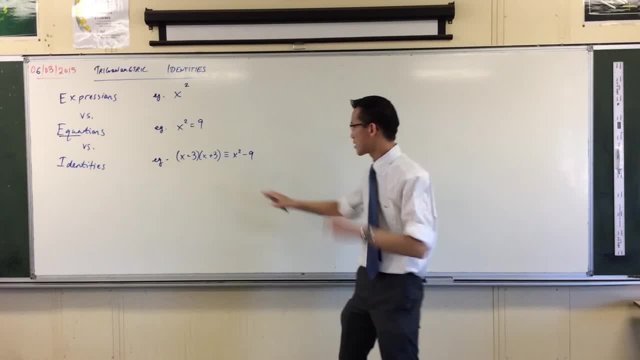 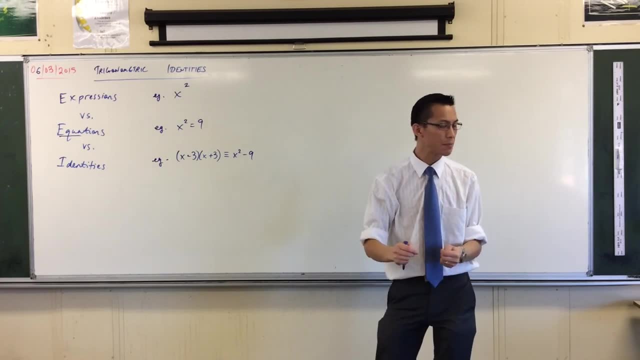 been writing. your trigonometry is just with an equal sign. okay, But this, like you're used to this, in the context of like triangles and all that kind of thing, we associate this with congruence right Now. congruence is a good thing to connect it. 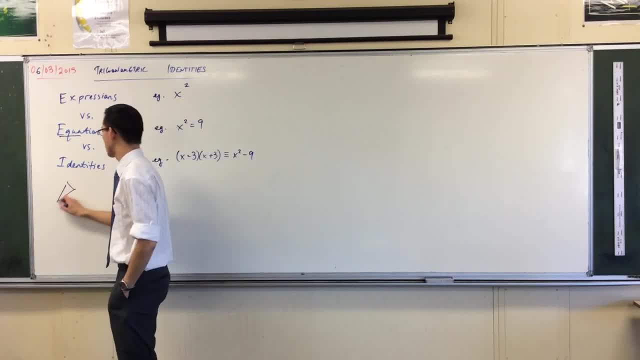 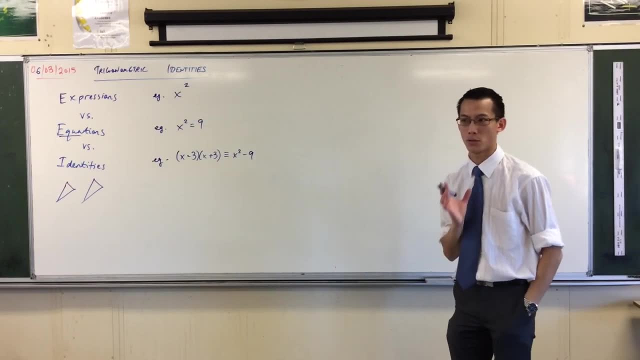 to, because when you've got two triangles and we say these two triangles are congruent, we mean that they are identical in every possible way: Same shape, same size, everything, Everything about them is the same, And that's the same thing that we have here. 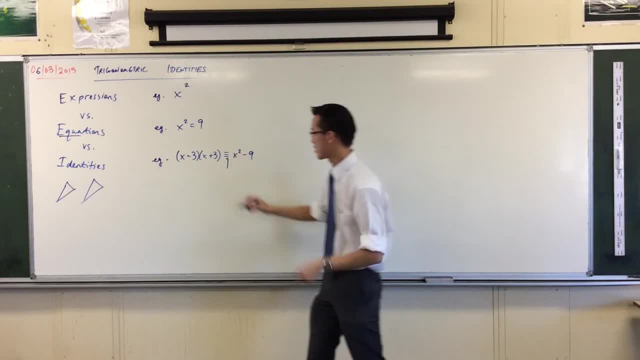 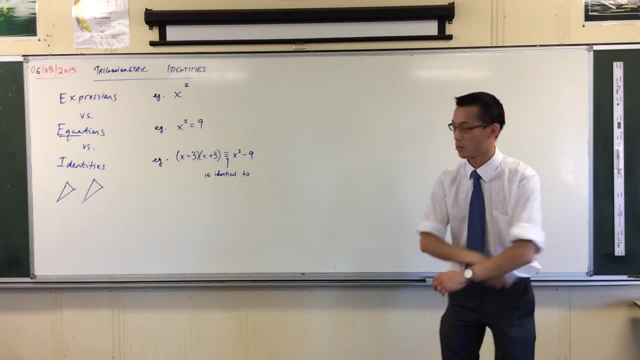 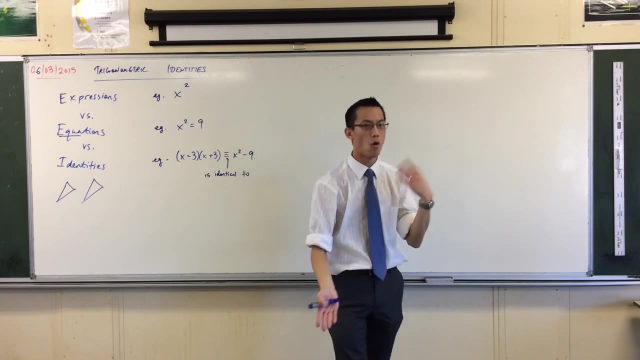 right. So I read this as in this context, I'd read it as: is identical to okay. As opposed to is equal to right. Now let's get at this another way. okay, This is an expression. Expressions cannot be true or false. okay, Because it's just a. 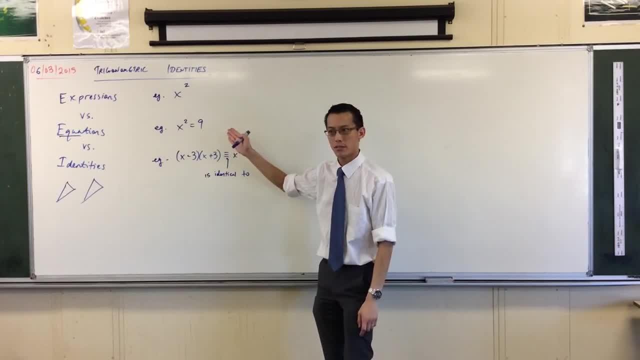 word that's out there. okay, An equation. an equation is only true if it's true sometimes, right, It's true, I should say, for it's true for certain values of x and it's not true for other values. okay, For instance, this equation is only 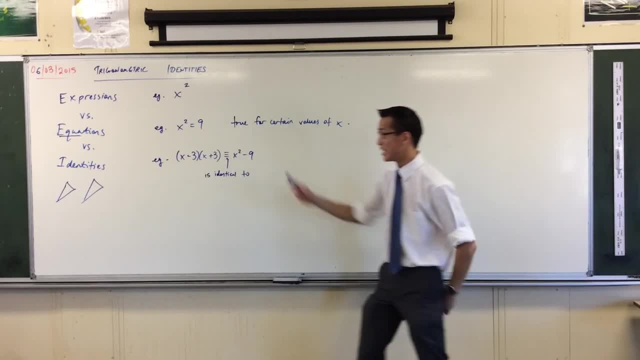 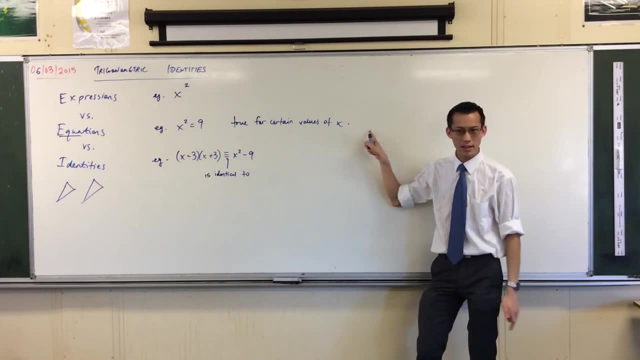 true for x equals plus or minus 3.. But if x equals 2, it's not true, It's a lie, right? It's only talking about very specific x. So this is true for certain values of x. It's true sometimes. 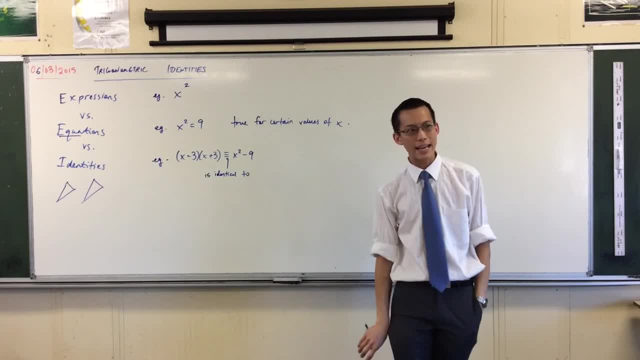 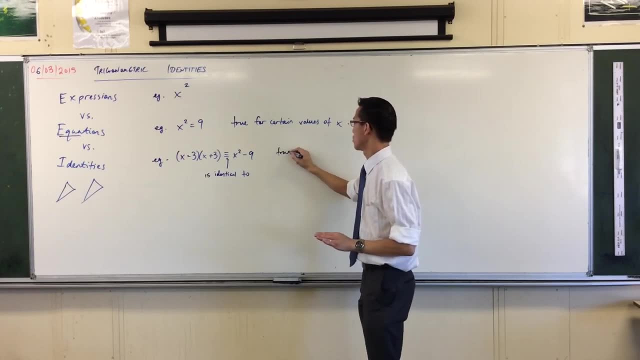 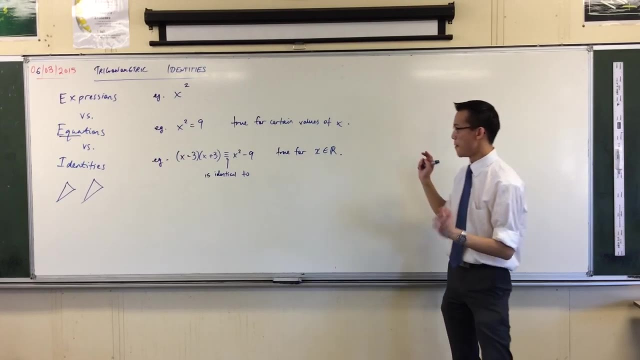 This, though: you can throw any x you like in there, and both sides will always be identical, So this is not true for certain values of x. This is true for all real values of x. okay, You can throw anything you like any day. This is true sometimes, but this is true. 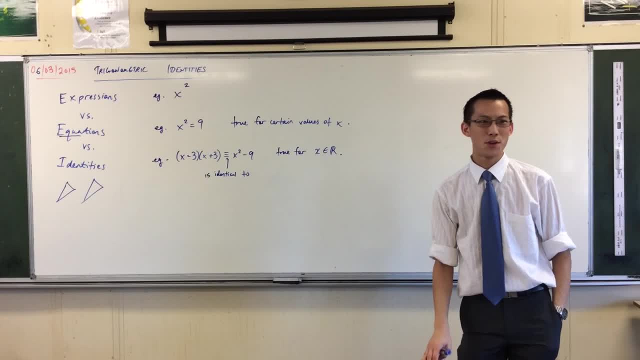 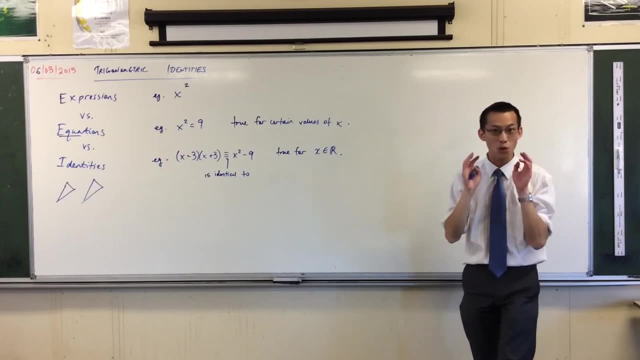 always okay. So let me give you a really cheesy way to remember this- Super cheesy, but I promise you'll remember it, okay. Equations, equations, identities. Let's put this all in English, okay. So an expression would be a word like say cool, That's just a word, It doesn't mean anything, It's not. 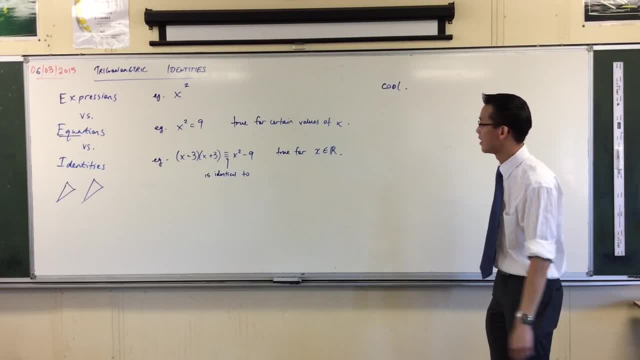 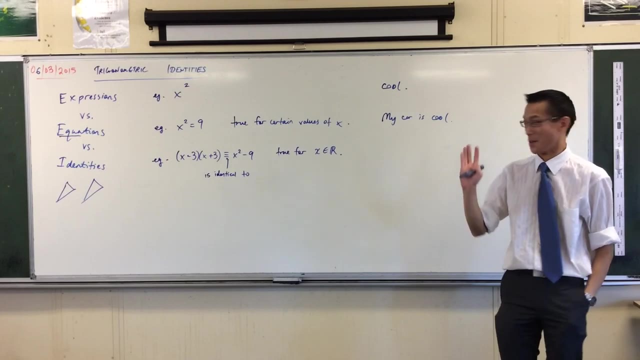 a statement Like it can't be true or false, It's just a word. okay, I could extend this and say: my car is cool, right? That's a statement of equality, right? Except it's only true some of the time, right, The air con in my car is terrible, so it's only true in winter.